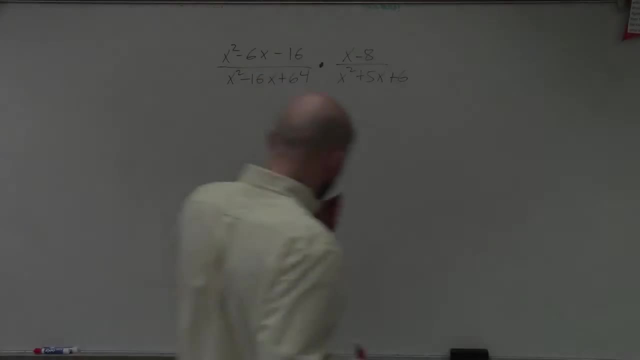 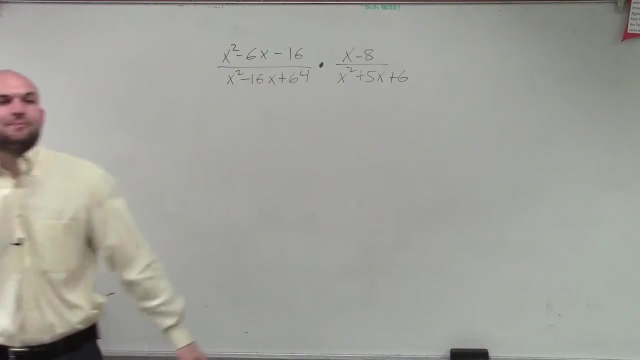 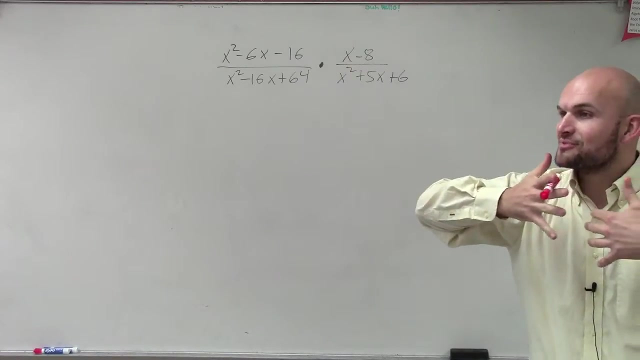 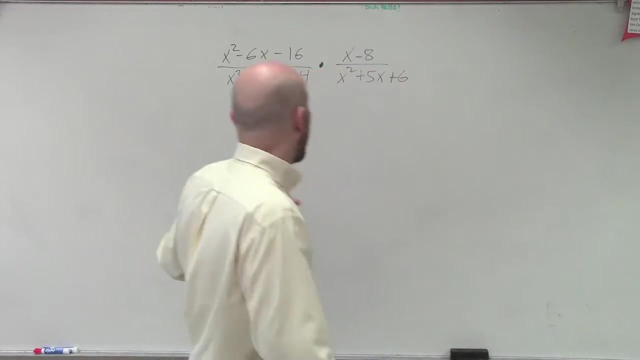 All right. so whoa lost my marker? In this example, ladies and gentlemen, we have a fraction times another fraction. So we know, in fractions times fractions, we just multiply across right Now. I, you know, might be a little crazy here once in a while, but I'm pretty. 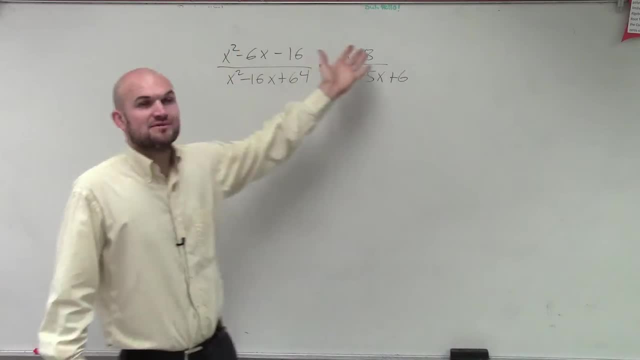 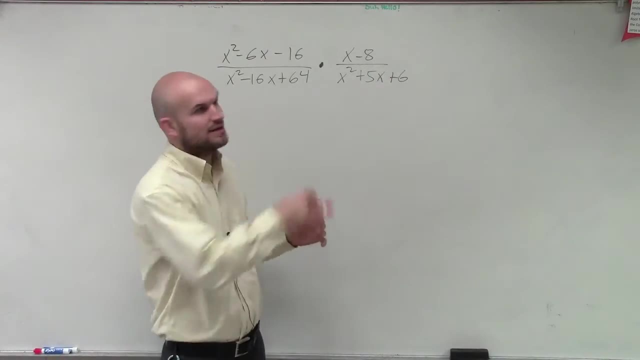 sure I don't want to multiply my trinomial times a binomial, because I have had to do that before Christian and it was not very much fun. Yeah, yeah, yeah, that means you're supposed to be writing this one down. That's awesome. And then I know. well, then you. 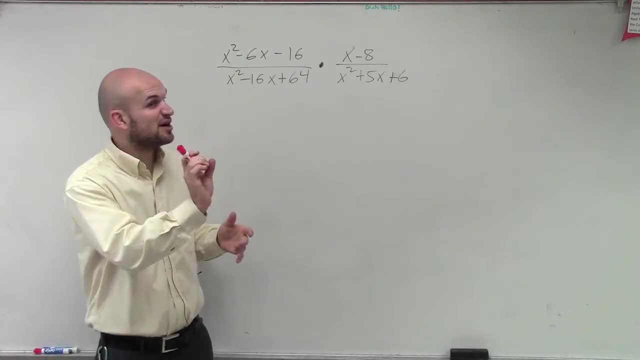 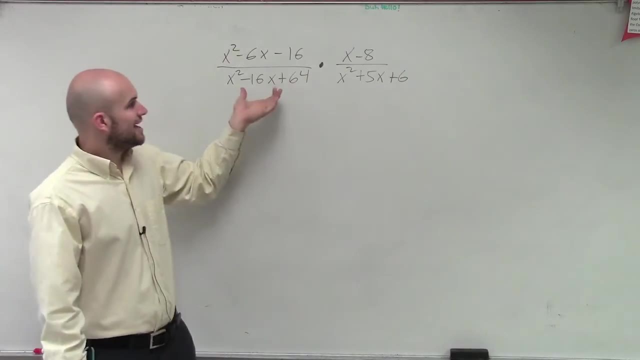 want to be watching what we're going to do there, because it's going to become very important, because if you multiply this times, this, we can do it. We've learned how to do it, It's possible. Then you have a trinomial times, another trinomial. That's going to be a lot. 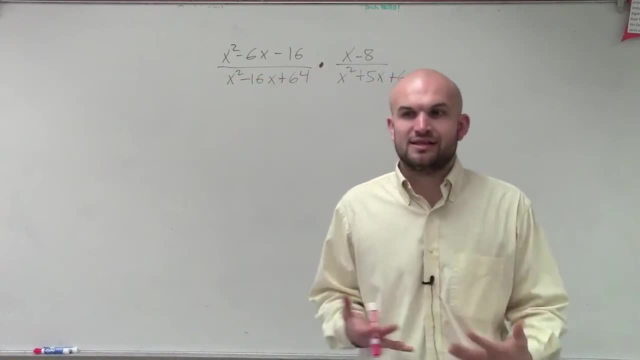 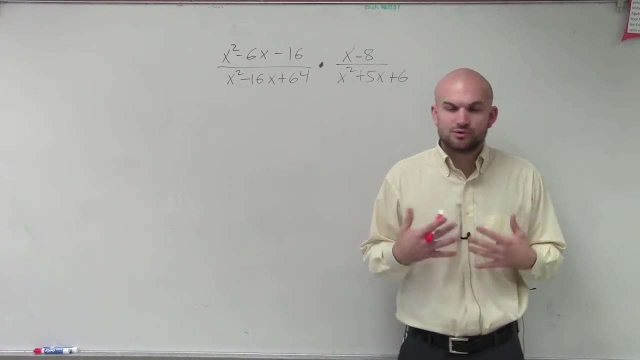 of work as well. So what we want to do is, before we do that, we want to do a little before we multiply any of these out, since we have polynomials, let's see if we can simplify this any further to undo or to eliminate some of our common factors. So the first, the main, 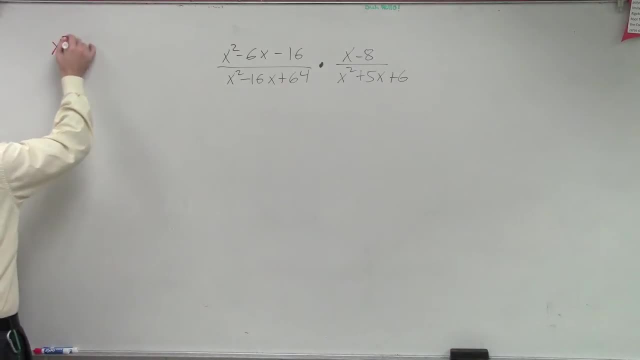 important thing, what I'm going to have you guys do. what I would just recommend is, if you guys are really good with your factoring, then you can just factor on the problem on your separate sheet of paper. If you're not very strong in factoring, you're probably 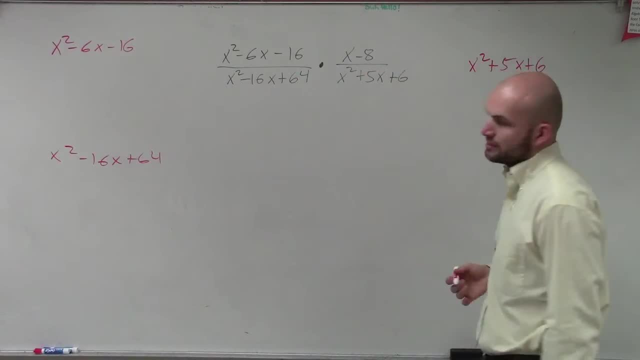 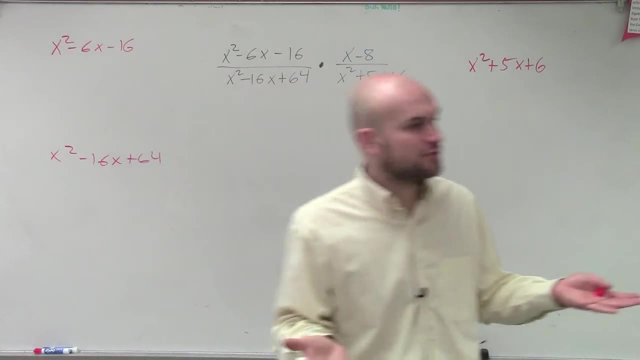 going to want to write out each term that you can factor. Now, in this case, we all have trinomials, we can factor, but you guys, as you know, you can factor out a binomial, right? If you had a binomial of 3x plus 6, you can factor out. 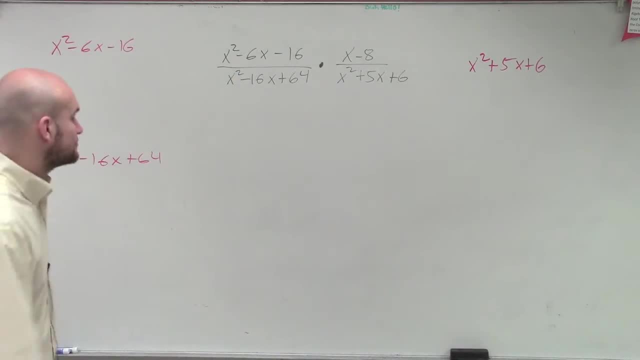 a 3, right, So it's anything you guys can factor. So here I have x squared minus 16x minus 16, so I want to see, can I factor this? The factored form is x minus 8 times x plus. 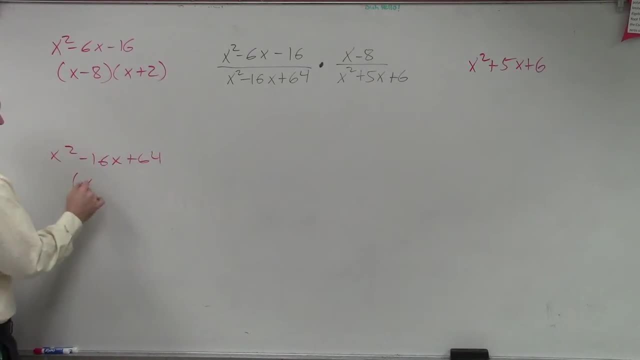 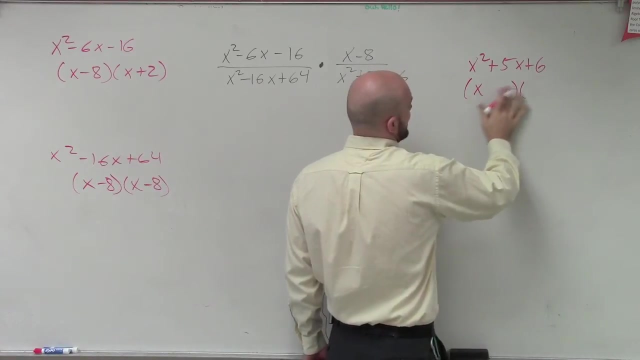 2,. right Here, what can I factor? This is a perfect square trinomial, which hopefully everybody knows. Then we have this one, which would be x plus 6,. no, no, x plus 5,, x plus 3,, x plus 2,, okay. 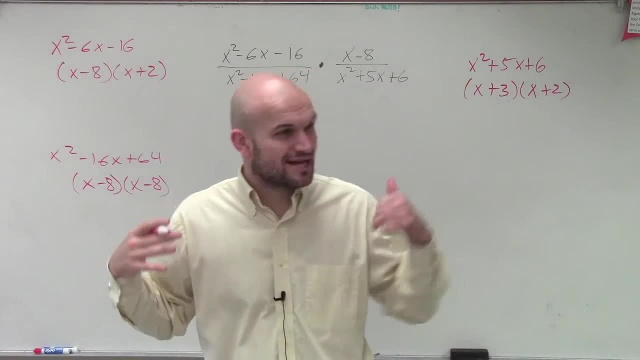 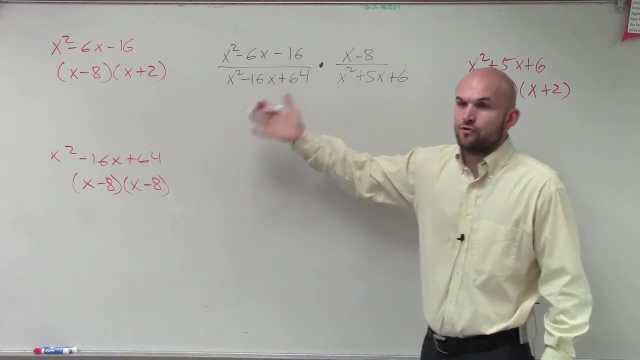 So now all I'm simply going to do- do you guys see how I factored this out? It wasn't anything crazy, it's stuff we've already done. But now what I'm going to do is I'm going to substitute in our factored forms for each one of our polynomials that we have. okay, 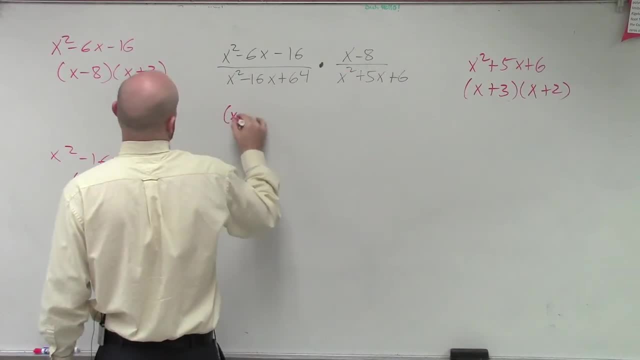 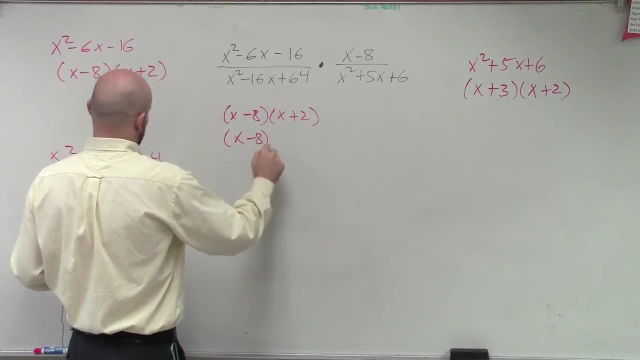 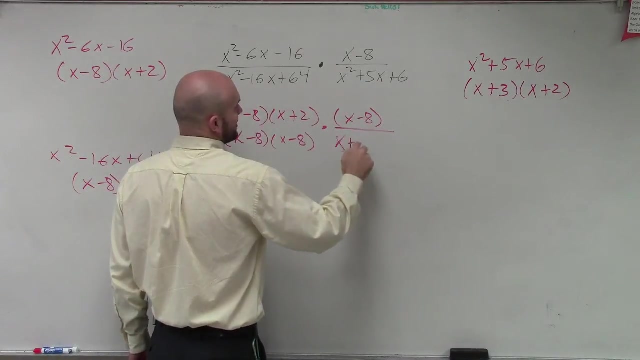 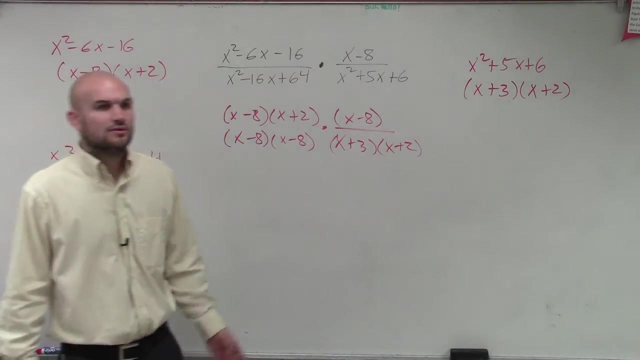 Now. so I have x minus 8 times x plus 2, divided by x minus 8 times x minus 8 times x minus 8, over x plus 3 times x plus 2.. Now when I'm multiplying across, ladies and gentlemen, 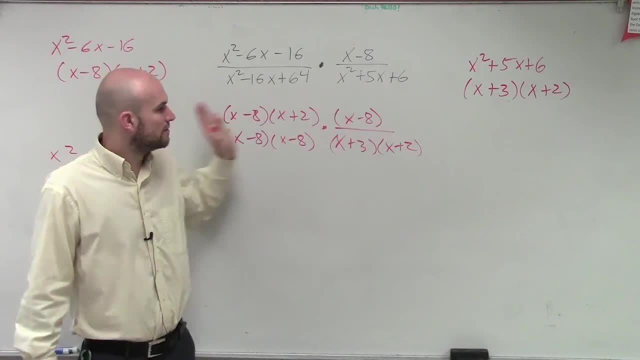 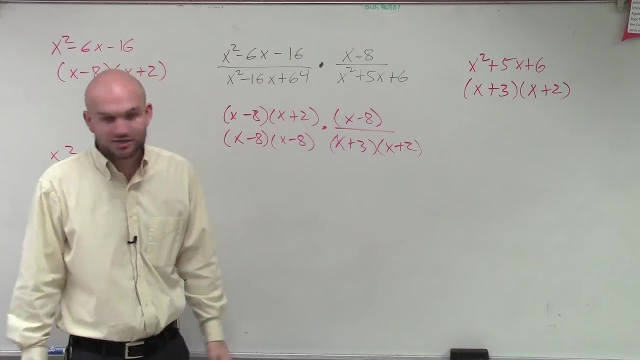 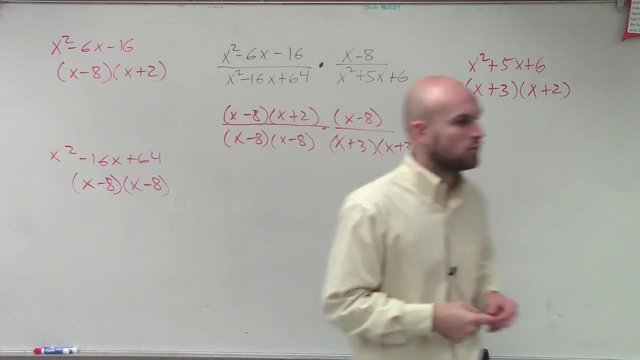 I'm multiplying everything across, right, Really, this all turns into: I'm multiplying this times this, and then this times this, so everything turns into a big multiplication problem. Everything's just a big multiplication problem. So now I need to see what terms or what factors or binomials can I now divide? 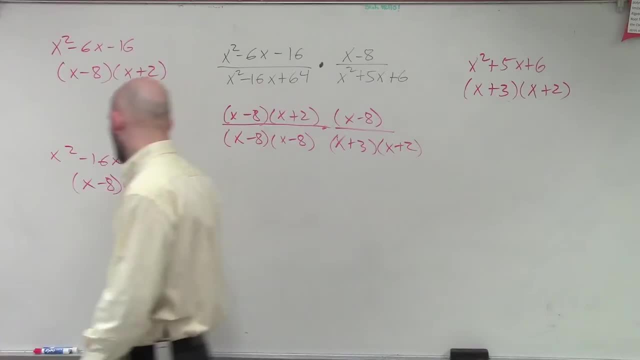 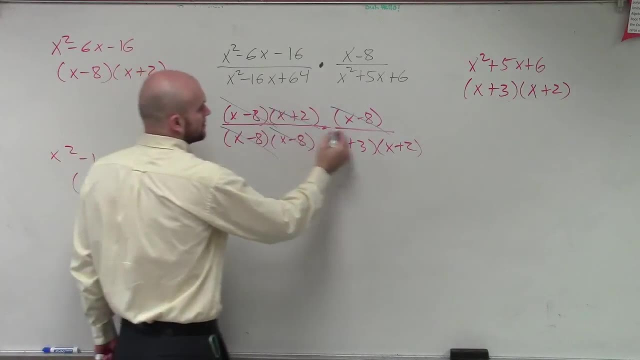 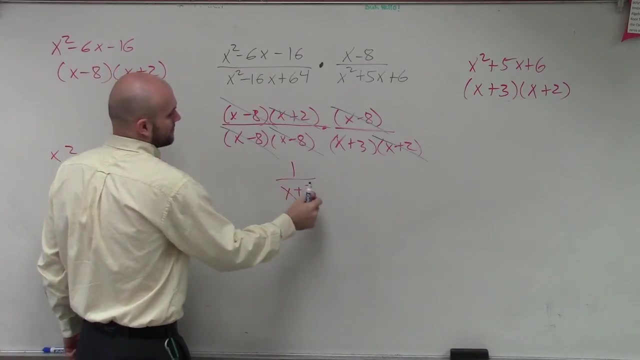 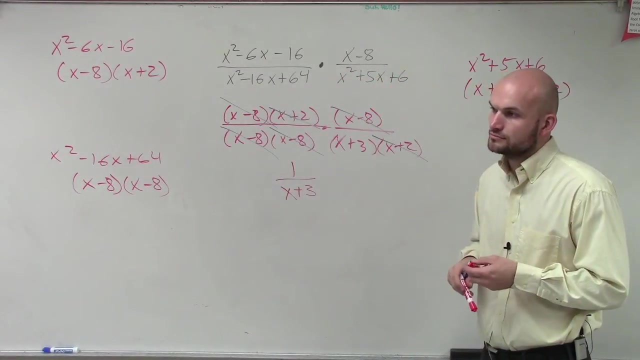 out, meaning divide, to give me equal 1?? Well, I see, those divide out, those divide out. Okay, both divide out, so I'm just left with one over x plus three. I did that last time. They can divide out even though they're split down.